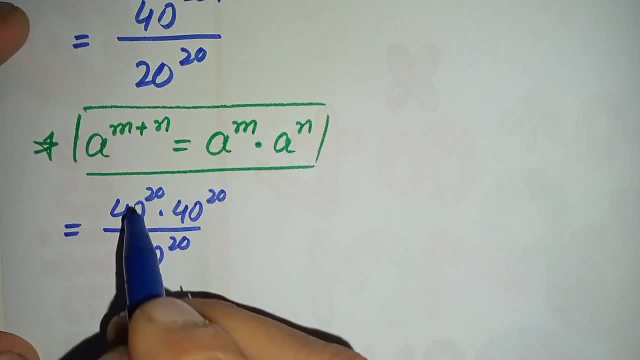 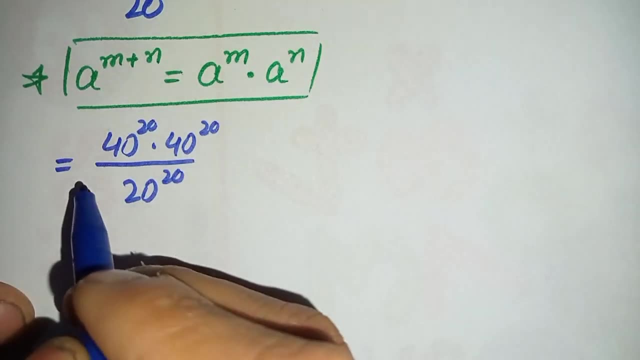 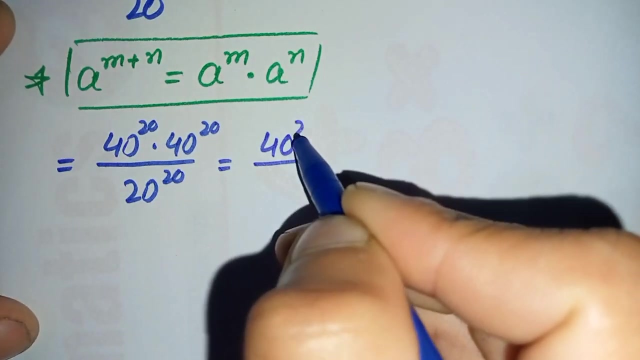 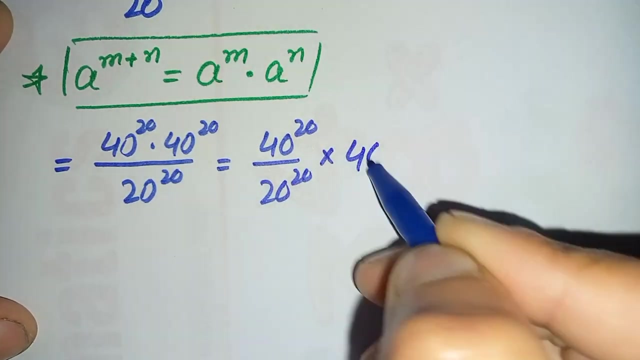 power 20. now, in the next step, these two numbers has the same power. so here we will split this number from the division of these two numbers, so we can write this further, as is equal to 40 raised to power 20 divided by 20 raised to power 20. multiply 40 to power 20. look into these. 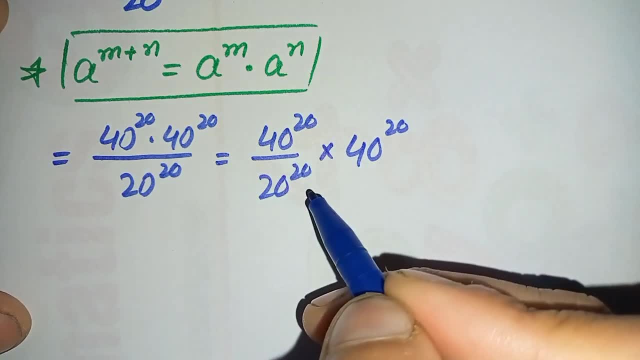 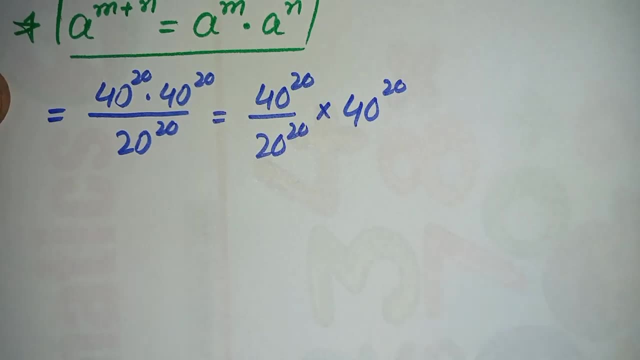 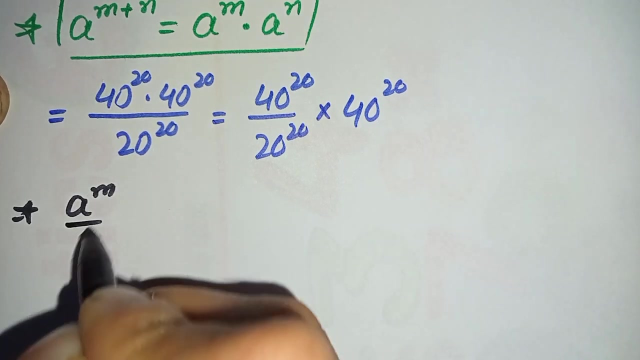 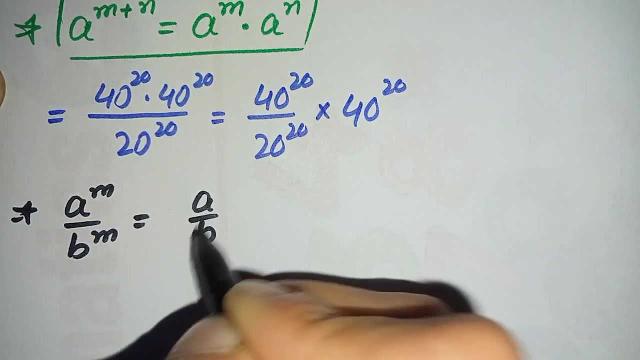 two numbers in the numerator and denominator. both the number has the same power: 20. so here we will use the same power. explanation: math property. so here we will use this one property: a raise to power 20. m divided by b raised to power m can also be written as a by b or less to power m. 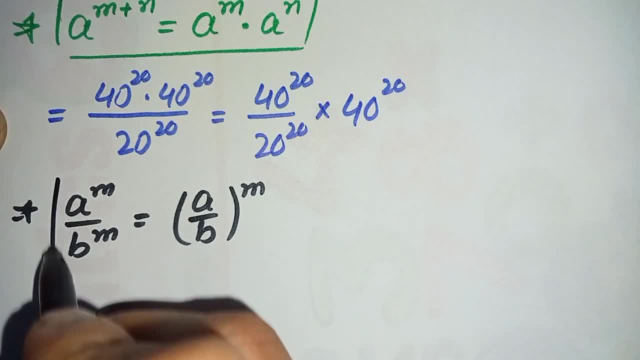 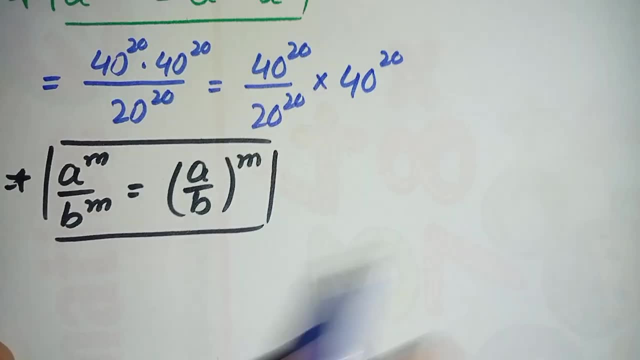 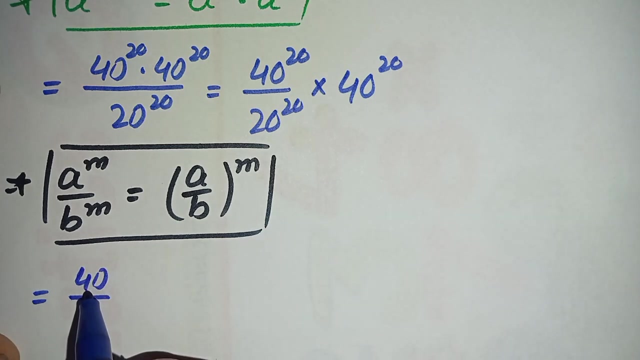 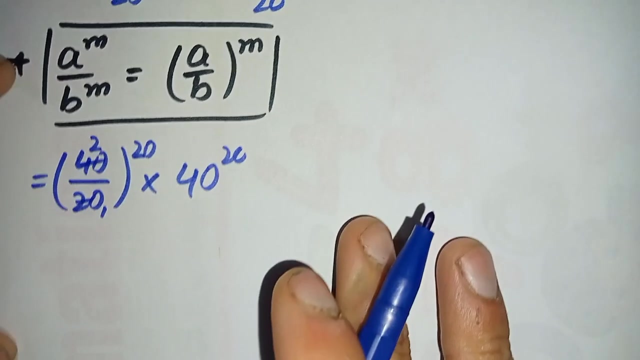 where a, b are any two real numbers. so using this exponential property of the same power here in this equation it will become- from here we will take the power common, it will become 40 divided by 20. whole raise to power 2 x 20. My guess it was not 2, it was 20, so next it will become 2 by 1 is equal to 2 will. 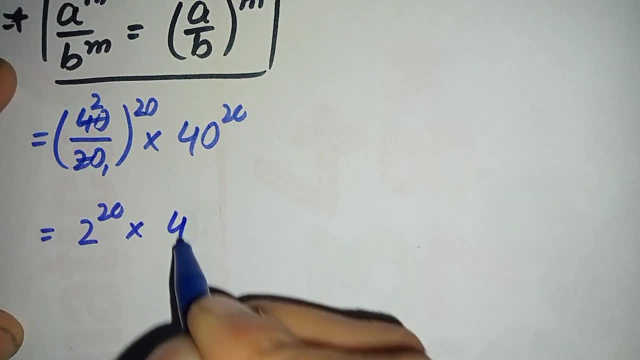 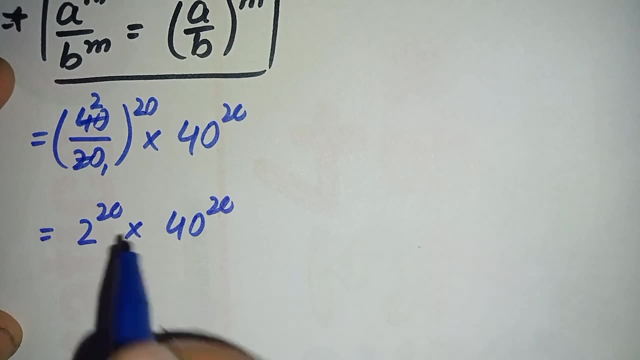 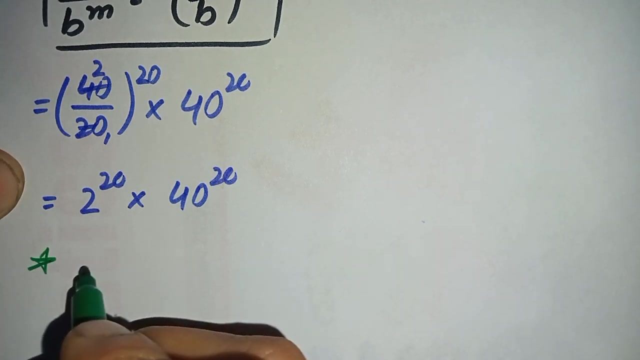 become 2 raised to power: 20 x 40. raised to power: 20. Now look at two, these two numbers. bli number says the same power. so here we will use the same power to the product formula. so here you will use this one result: a raise to power m times b raise to. 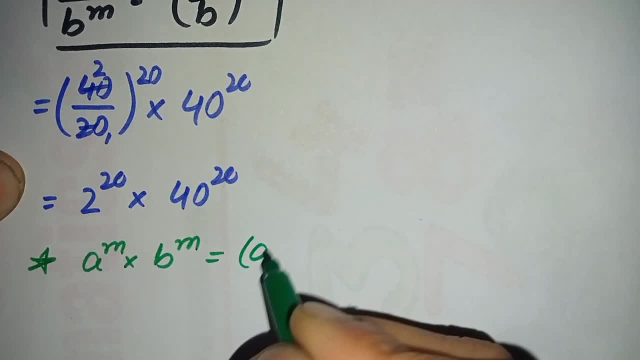 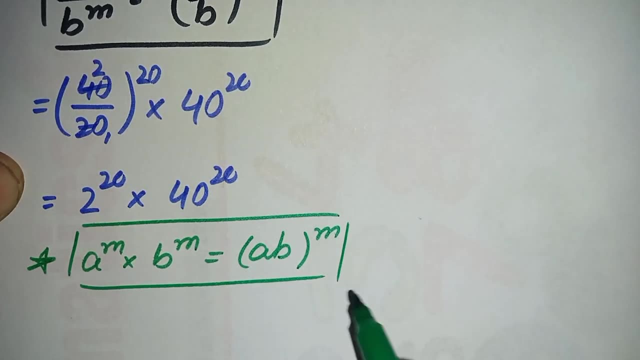 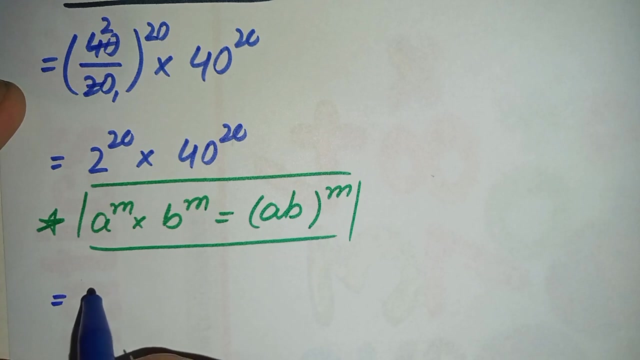 power m can also be written as a times b whole raise to power m where a, b are any two real numbers. so using this result here in this equation- this equation will become here- we multiply the basis and we will take the power out in common. so it: